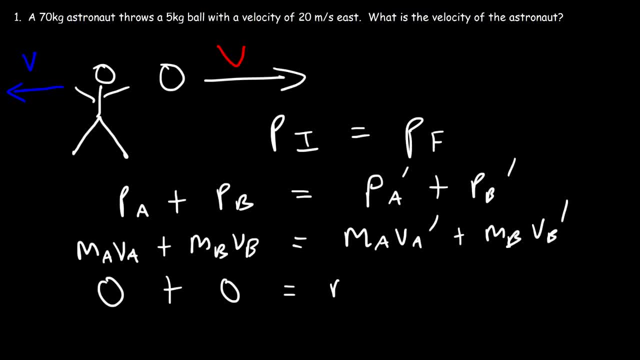 momentum. So therefore we have this equation: Zero is equal to MAVA plus MBVB, So I'm going to take this term and move it to this side. So negative MAVA prime, which stands for final velocity, is equal to MBVB prime. 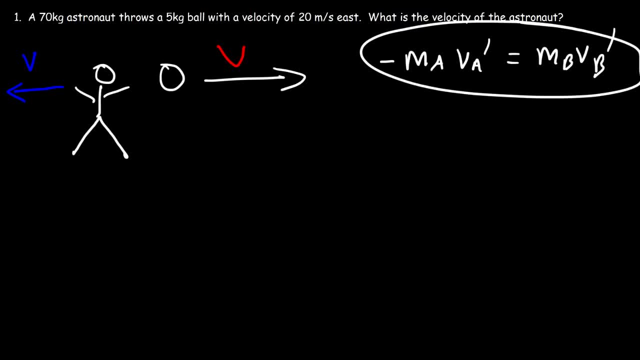 So let's plug in what we know Now. the mass of the astronaut is 70 kilograms And we're looking for the velocity of the astronaut after he throws the ball. The mass of the ball is five kilograms. The velocity of the ball is positive, 20.. It's positive because 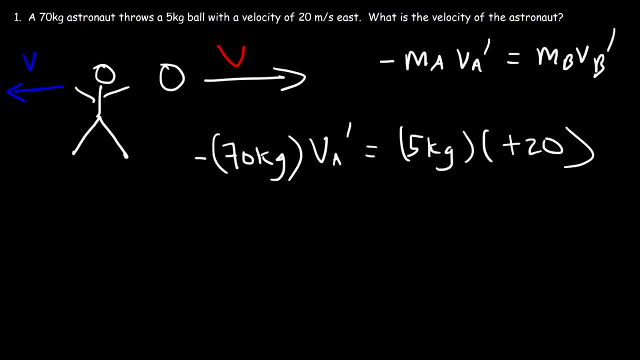 the ball is moving towards the right in the positive x direction. So this is going to be 5 times 20, which is 100.. So we get negative 70VA prime. prime is equal to 100. now we get a divide both sides by negative 70, so the 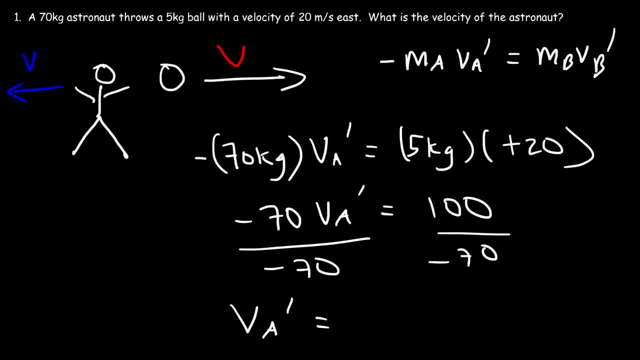 final velocity, the astronaut is negative: 1.43 meters per second. now the reason why the answer is negative is because he's moving in the negative X direction. now notice that the velocity of the ball is significantly greater than the velocity of the astronaut. because the astronaut has more mass, he's gonna move. 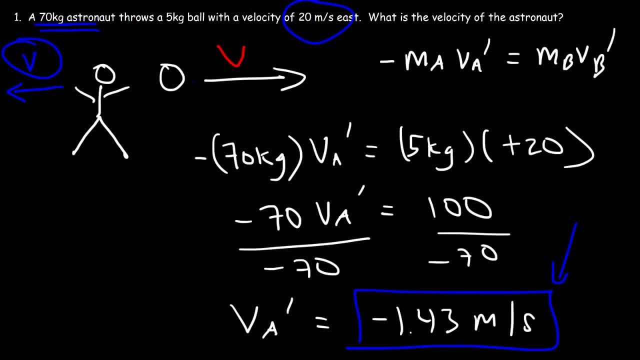 backward with a lower speed. the ball has less mass than the astronaut, so it's gonna move to the right with a greater velocity. so as the mass increases, the velocity decreases, assuming if the momentum is constant, if it's conserved. if you decrease the mass, the velocity increases. 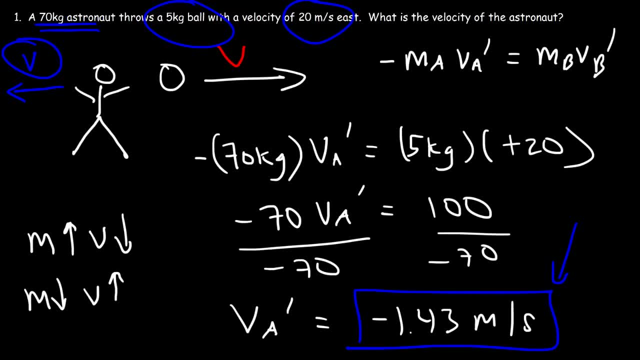 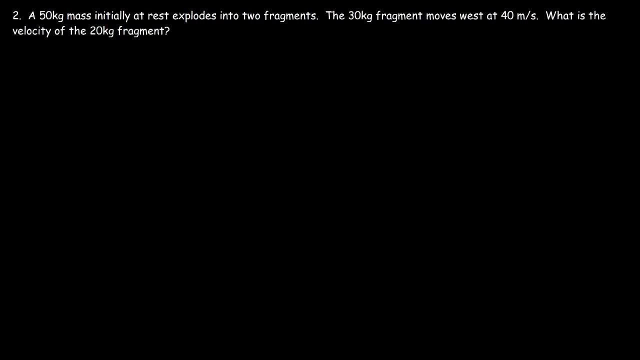 so whenever momentum is constant, objects with a very large mass tend to move slower, and objects with a low mass, objects that tend to be light, are the ones that move faster. now here's another similar question. a 50 kilogram mass, initially at rest, explodes into two fragments. so let's say this is the 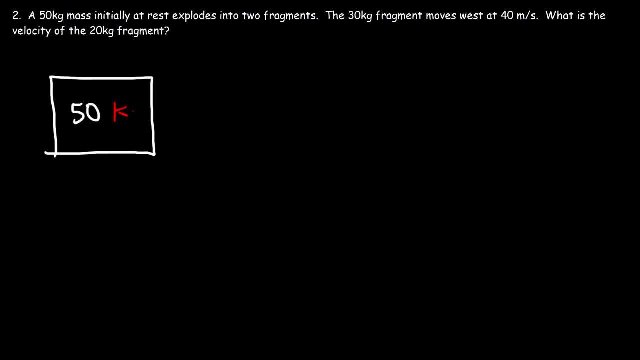 50 kilogram object. then after some time period it explodes into two parts. so let's say: this is the first fragment and this is the second fragment. now the 30 kilogram fragment that's going to move West at 40 meters per second and our goal is to find the зв. 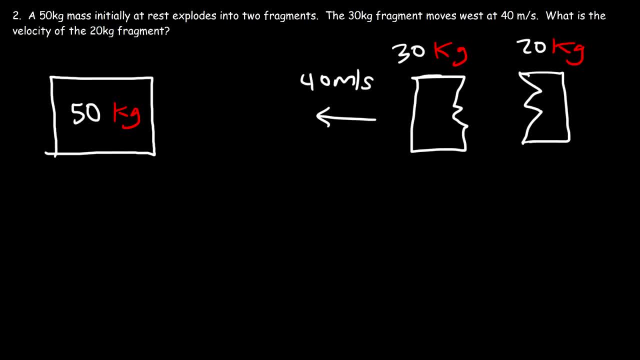 the velocity of the 20 kilogram fragment. Now we know it has to move east, so the velocity has to be positive. So once again we have: the total initial momentum is equal to the total final momentum. Before the event, this object was at rest. 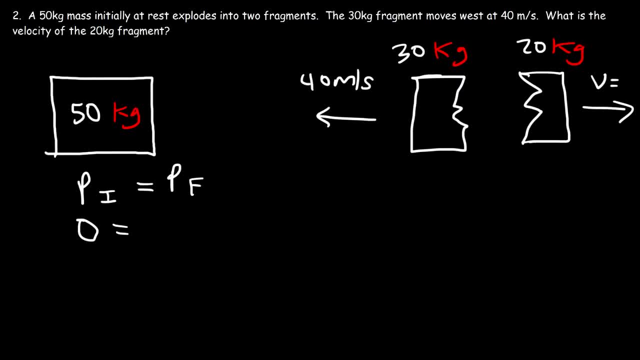 so the total initial momentum is 0 and the final momentum is going to be the momentum of the first fragment plus the momentum of the second fragment after the collision. So let's call this fragment A and fragment B. So, just like before, we're going to have this equation: negative MA, VA prime is equal to MB VB. 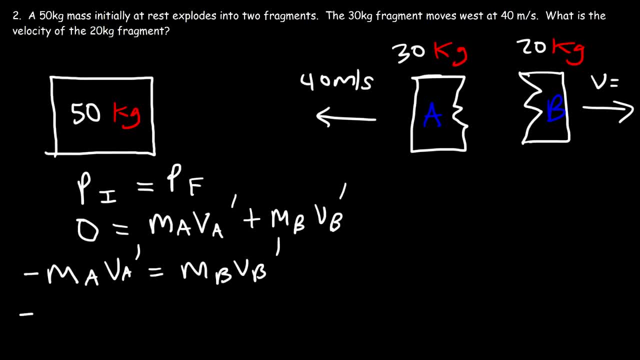 prime. So fragment A has a mass of 30 kilograms and the velocity of negative 40. Now you need to put the sign of the velocity, because this is moving to the west, so it has a negative value. The mass of the second fragment, fragment B, is 20 and we need to calculate VB. 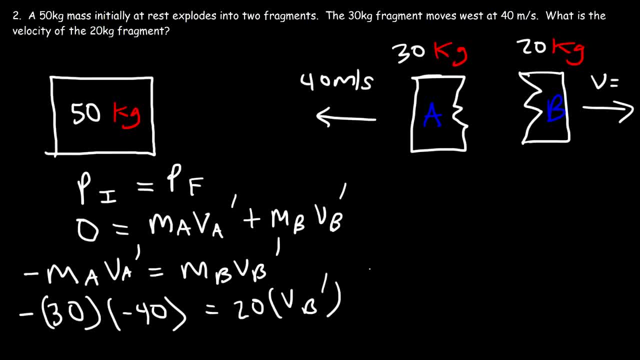 So negative 30 times negative 40 is positive 1200 and that's equal to 20 times VB prime. So 1200 divided by 20 is 60 and we have a positive answer to indicate that it's going east in the positive x direction. 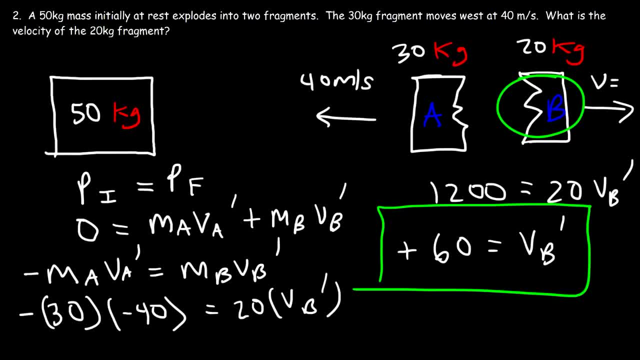 So that's the final velocity of fragment B. Now, fragment B has less mass than fragment A, and therefore fragment B has a greater speed. Fragment A has more mass and so the speed is less: it's 40 meters per second as opposed to 60 meters per second. 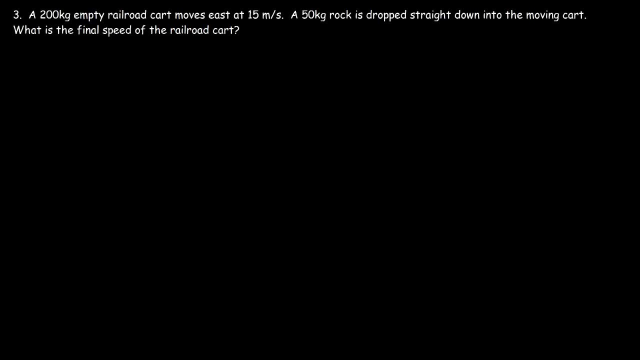 Now let's move on to our next problem. A 200 kilogram empty railroad cart moves east at 15 meters per second. A 50 kilogram rock is dropped straight down into the moving cart. What is the final speed of the railroad cart? 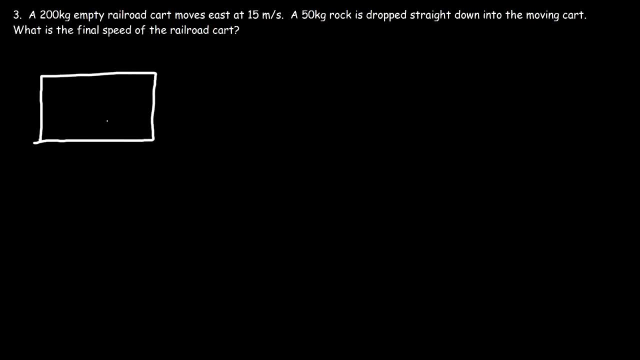 So let's say this is the cart. It has a mass of 200 kilograms and it's currently moving at a speed of 15 meters per second. Now what's going to be the new speed if we take a rock and drop it into it? 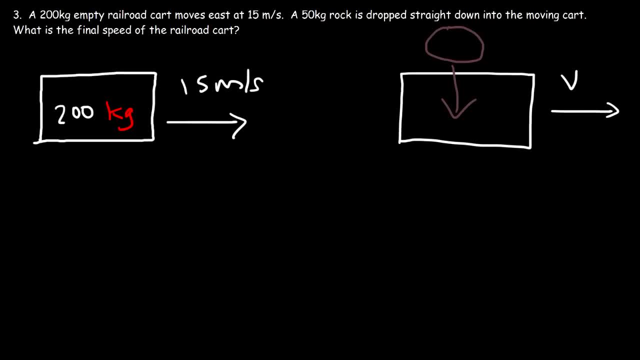 Now the momentum of this object in the x direction is fixed and this rock is moving in the negative y direction, so it's not going to affect the momentum of this cart in the x direction. So the momentum is going to be conserved. Now, if the momentum is constant and if the mass increases by, in this case, adding the 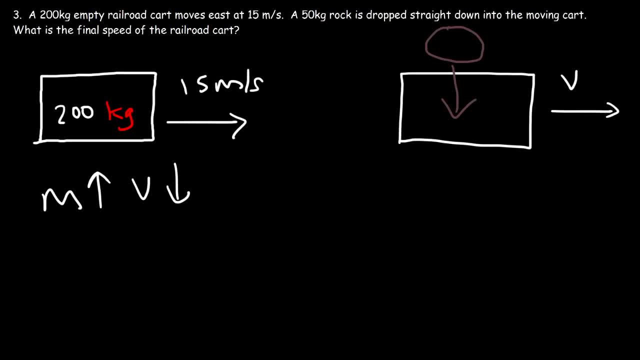 rock, we shall expect that the speed should decrease, So our answer should be less than 15.. Alright, Let's do it. Okay that we had before. P initial has to equal the momentum after P, final, so let's calculate the initial momentum. it's going to be mass times velocity, so 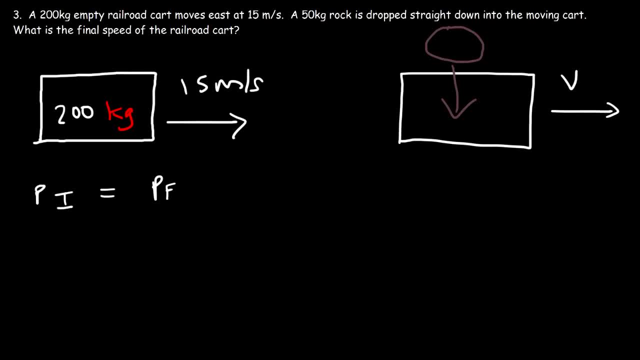 that's 200 times 15, so that's 3000. now that should equal the final momentum, so that's MV. now the new mass is no longer 200. it's the 200 kilograms of the railroad cart plus 50 kilograms of the rock. so the total mass of this object. 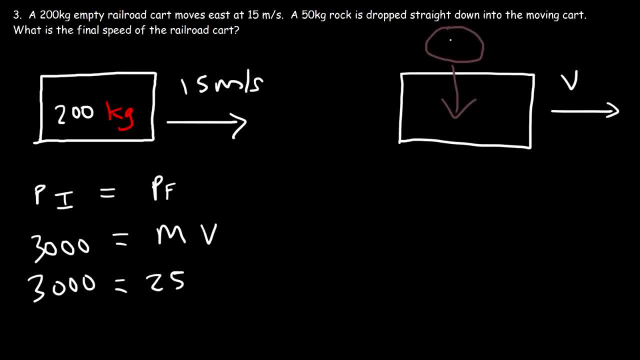 now this system is going to be 250 kilograms, and now we got to calculate the new speed. so it's 3000 divided by 250, and so the railroad cart with the rock is going to move at a combined speed of 12 meters per second. so now let's talk about what's happening here. so what? 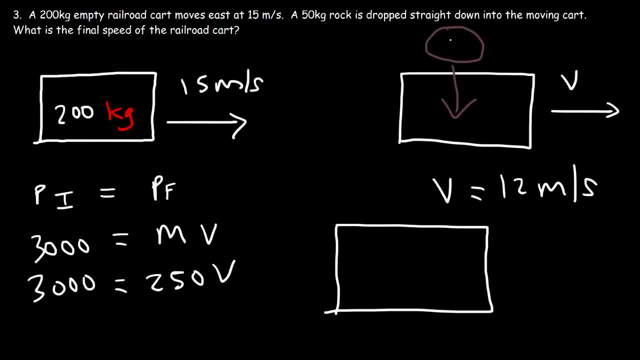 happens as soon as the rock falls into the cart. so let's say: this is the rock. now the speed of the rock in the x-direction initially was 0, now it's 12. so the rock accelerated in the x-direction since once you stop the rock, the rubble card is moving, and so this portion of 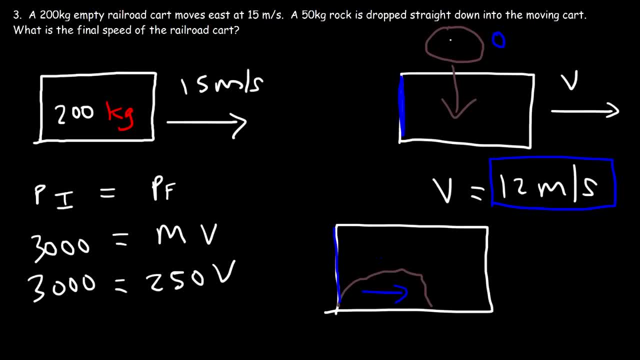 the rubble cart will exert a horizontal force on a rock, causing the rock to accelerate from 0 to 12 in the x-direction, now based on units. second law: for every action force there's an equal and opposite reaction force. so when the revel car exits a force on the rock, 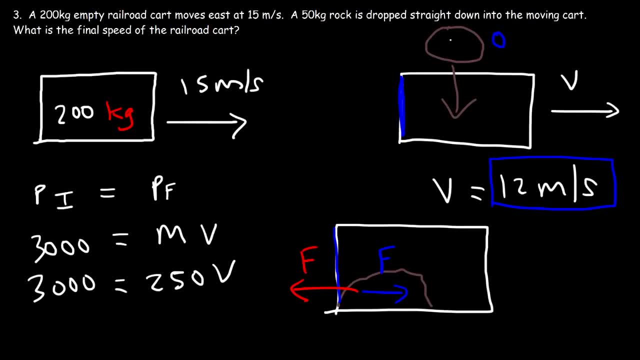 1, split x is 1. exerts a force on a railroad cart And so that force slows down a railroad cart from 15 meters per second to 12 meters per second. So that makes sense. The railroad cart accelerates the rock. 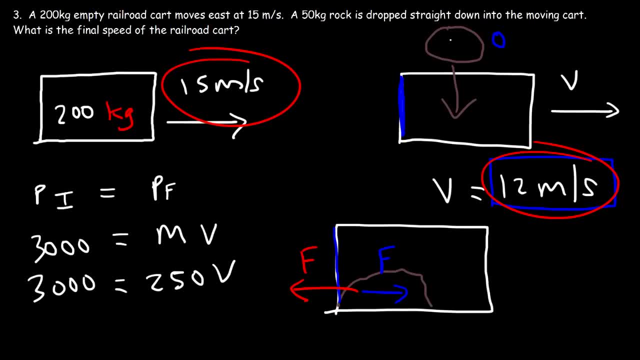 and the rock decelerates the railroad cart. But what's really happening here is that these forces are acting in such a way to transfer momentum from the railroad cart to the rock. If we calculate the new momentum of the railroad cart, the original momentum is 3000, but the new momentum is going. 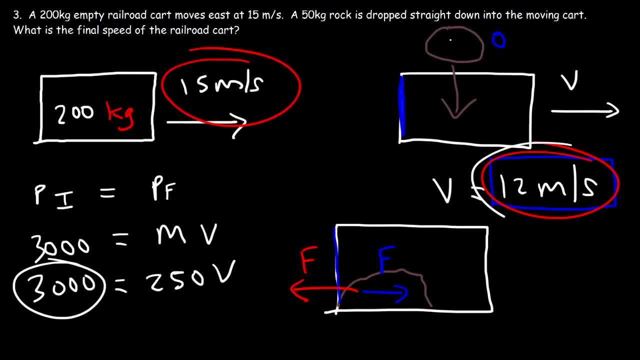 to be the mass of 200 times the final speed of 12.. So the railroad cart has a momentum of 2400, and the rock has a mass of 50 and a speed of 12.. 12: it's 50 times 12, which is 600. so the total momentum is still the same. so 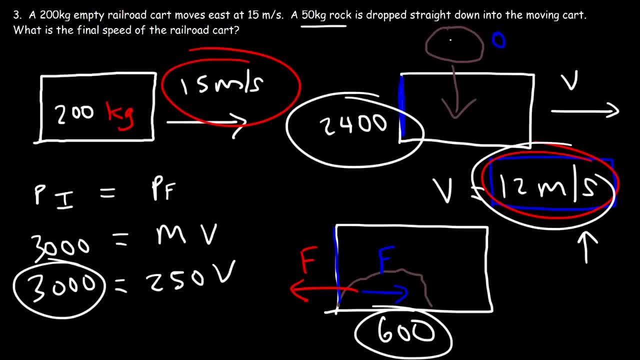 basically, the railroad cart lost 600 units of momentum and that 600 units was transferred to the rock. so these forces, they acted in such a way to take some of the momentum from the railroad cart and transfer it to the rock until the speeds of the rock and the cart were the same, until they reach equilibrium, so to speak.